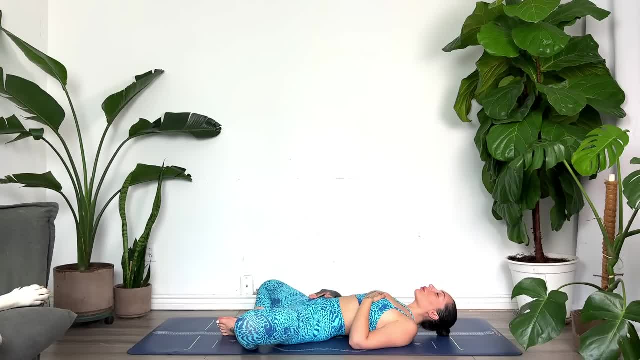 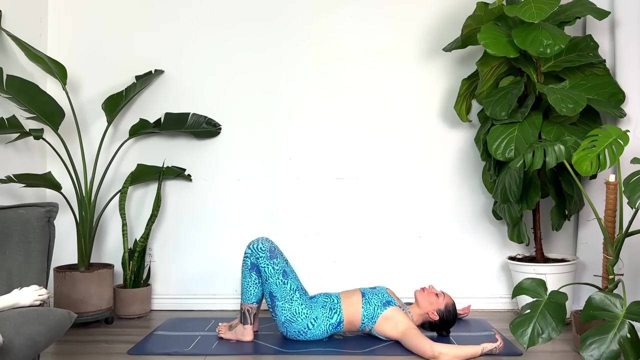 Gently lift the knees, taking the feet mat with distance. Begin to rock the knees gently side to side, rolling over the glutes and the lower back. Perfect. Allow both knees to fall to your left. Back stays flat on the mat for a supine twist. 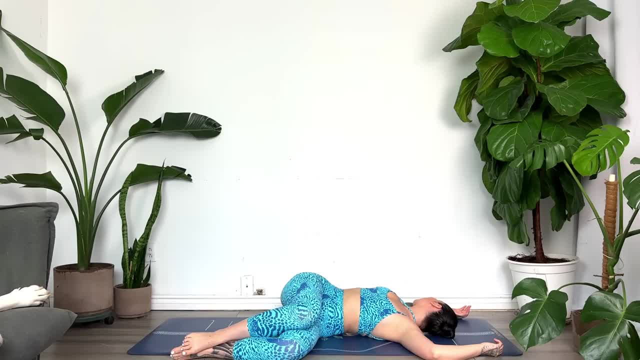 Option here to place pillows underneath the knees and or between the knees. for added height and support, You can also place a pillow or folded blanket underneath the right arm, the right shoulder- sorry for less of a twist. Utilizing your inhales to create space, maybe even feeling yourself lift as you breathe. 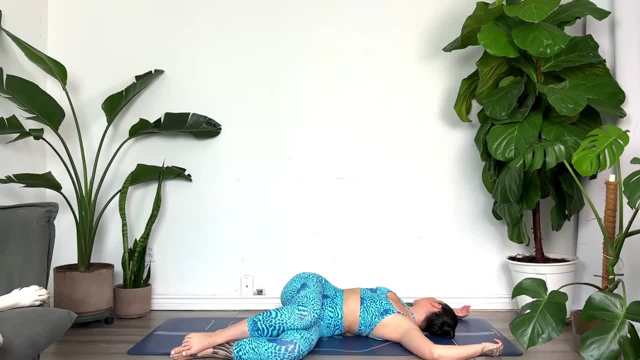 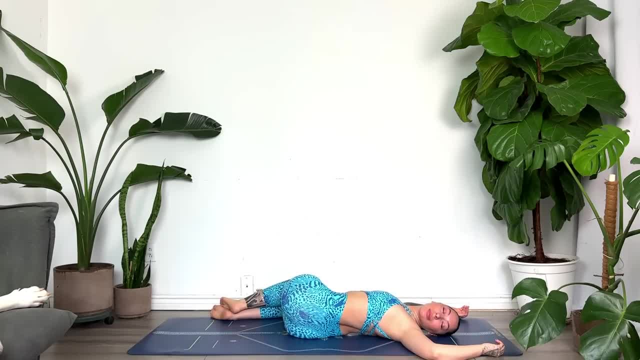 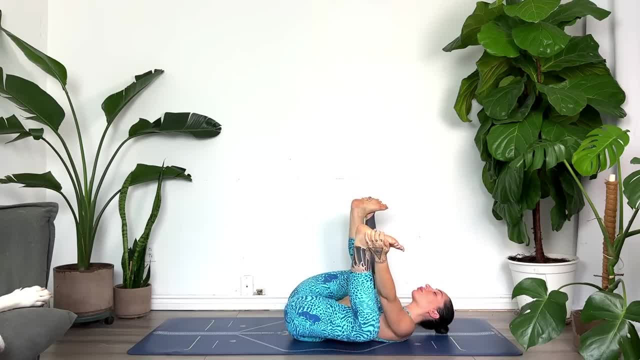 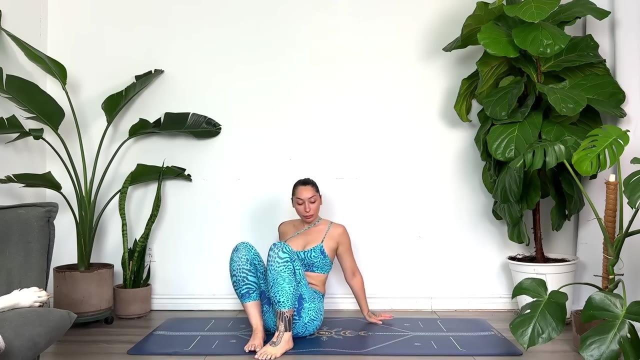 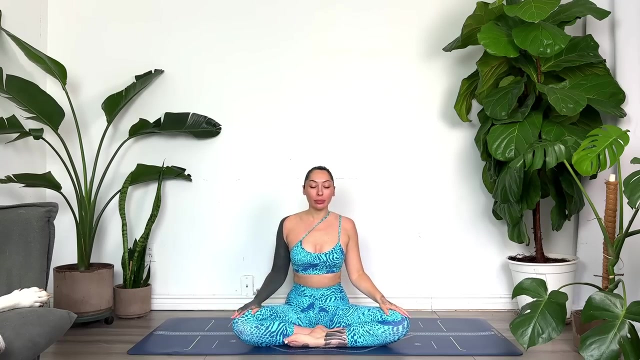 Giving your knees one last hug here and then we'll round up all the way to seated, whatever comfortable position that is for you, Finding some movement in the neck, feeling out all the clicks and ticks, maybe rocking the head forward and back. 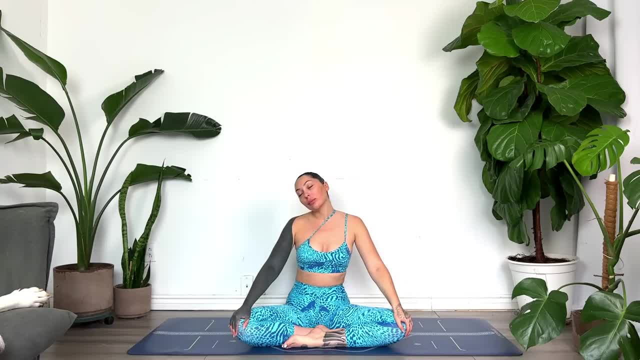 Side to side Again. whatever the body needs today, Sitting up nice and tall, take the left hand straight out to your left side and then we'll plant it on the mat. Staying here, draw the right ear towards the right shoulder. 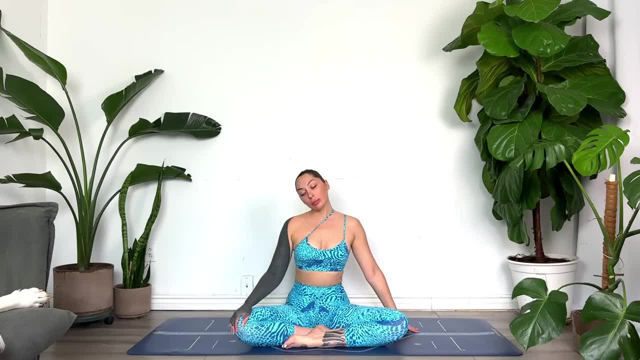 Option to find some movement, rocking the head forward and back, And we'll gently release, Shake it out and whenever you're ready, we'll switch sides, Staying wherever you feel most comfortable. Take your time. Your movement begins soon once FUCKING there. 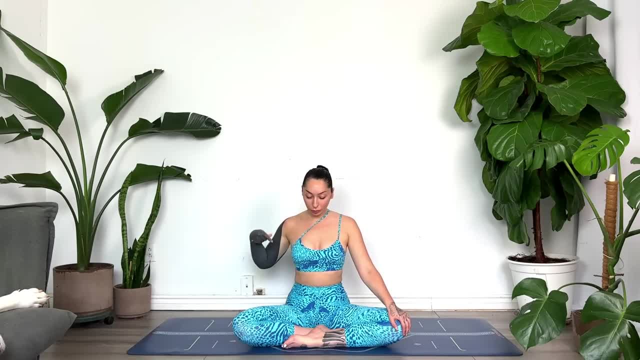 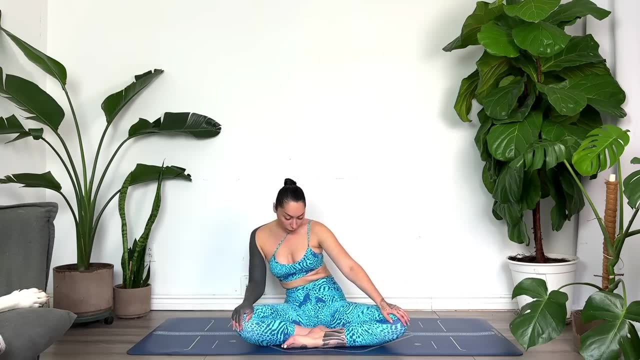 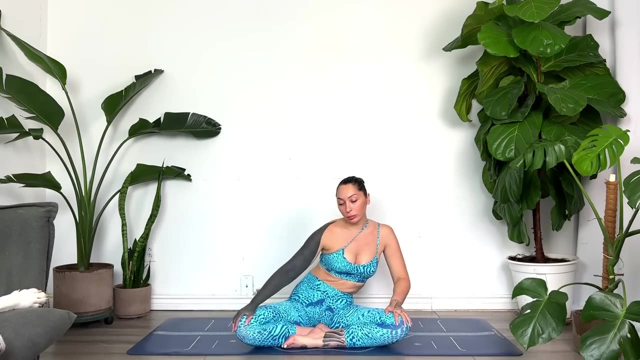 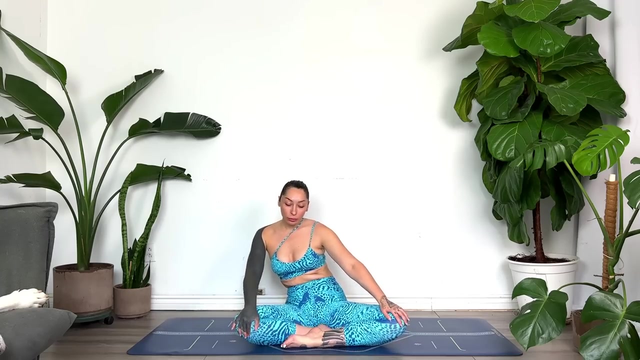 We'll slowly release Release. we'll begin to find some organic movement in the waste, just circling the waist or vielleicht même juste en tour d'reci: 320 g de cuivresse and rocking gently side to side. We'll come back to center, inhaling hands overhead. reach nice and tall. 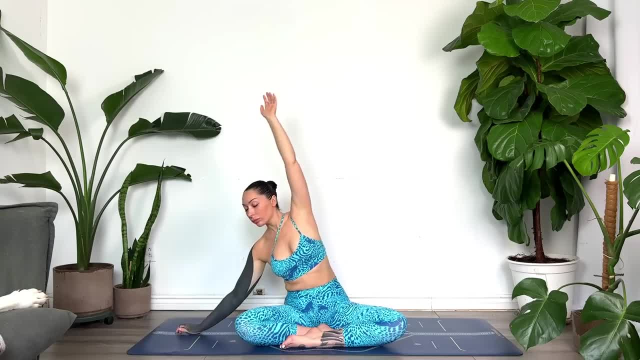 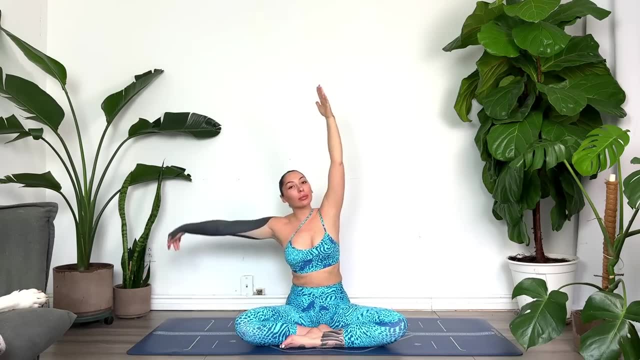 Exhale taking a side stretch towards the right. right hand to the mat. left hand reaches up and over option to come to the forearm. if that feels okay today, Inhale, reach back up. Exhale side stretch towards the left. 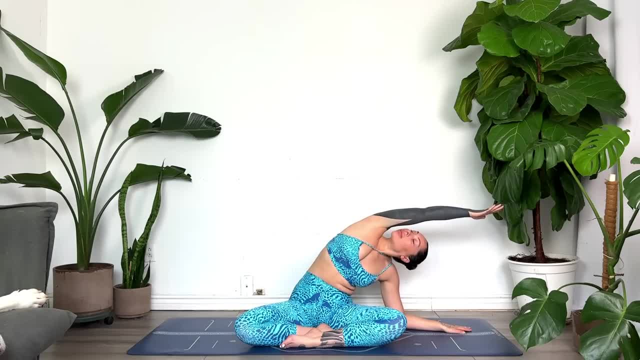 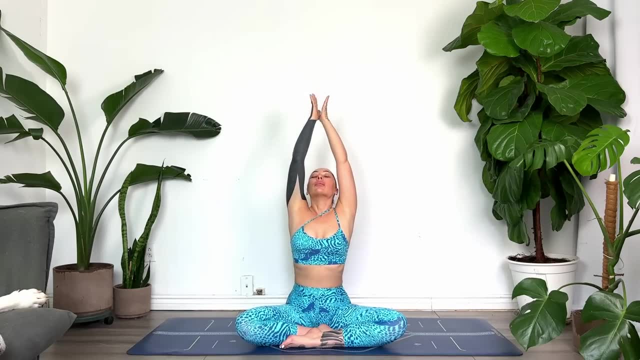 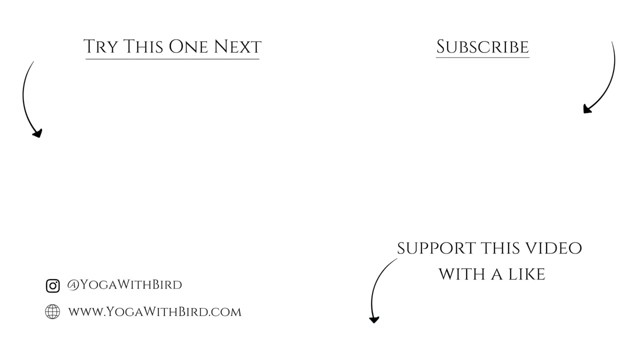 Inhale. reach back up Exhale heart center. Thank you for joining namaste.